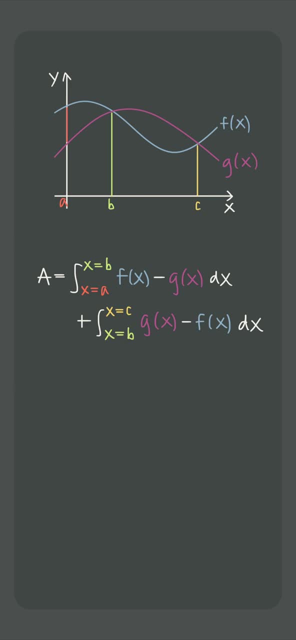 of g minus f over the interval b to c. This method always subtracts the lower curve from the upper curve, but we have to use a different integral between each intersection point. Alternatively, we can deal with the area in one piece, integrating over the entire interval. 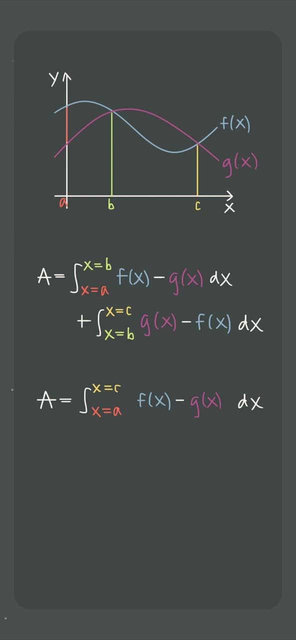 x equals a to x equals c all at once. We just have to take the absolute value of the difference of the functions. Both methods will produce the same value for area, so we can use either method. 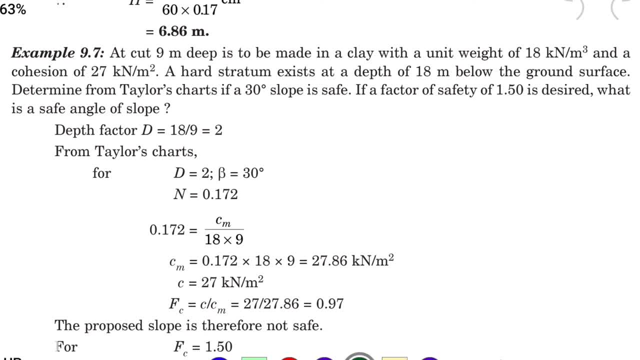 Hello friends, welcome to civil engineering exam. Today we are going to see the problem related with soil mechanics in the topic of stability of slopes. So the question is: a cut 9 meter deep is to be made in the clay with the unit weight of clay is 18 kilo Newton per meter cube. 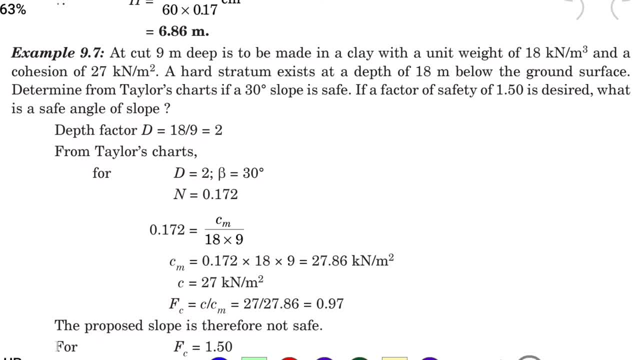 and a coefficient of 27 kilo Newton per meter square. A hot stratum exists at the depth of 18 meter below the ground surface. then determine from the Taylor's chart: if your angle is 30 degree, slope is safe. if the factor of safety is 1.5 is decide what is the angle of slope. so the first 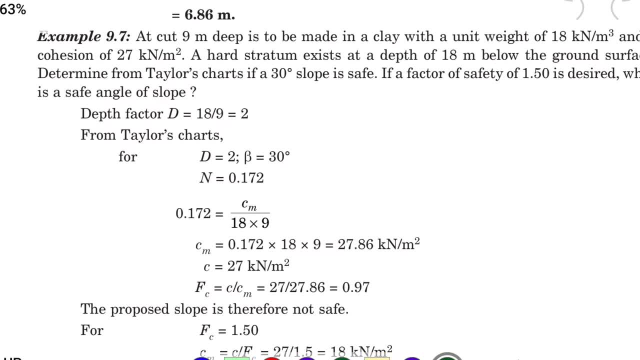 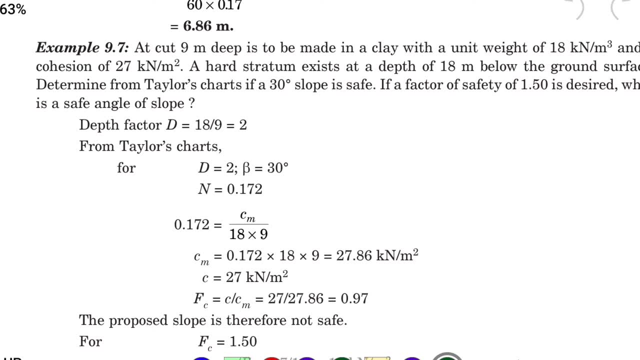 we have to find out. the depth factor d is equal to 18 by 9, so the 18 is depth is 18 meter below the ground surface and deep is 9 meter. the cut is 9 meter, so 18 by 9 equal to 2.. So from the 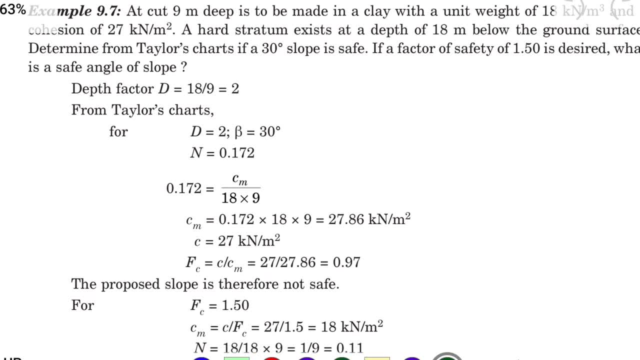 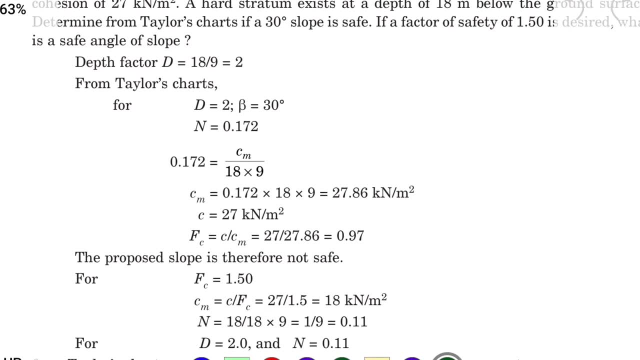 Taylor's chart, d equal to 2 and beta angle is 30. That is given. so for that n values we can take n equal to 0.172. so now we know the formula: n equal to cm divided by gamma into h. so now cm equal to the n values, 0.172 and gamma values. 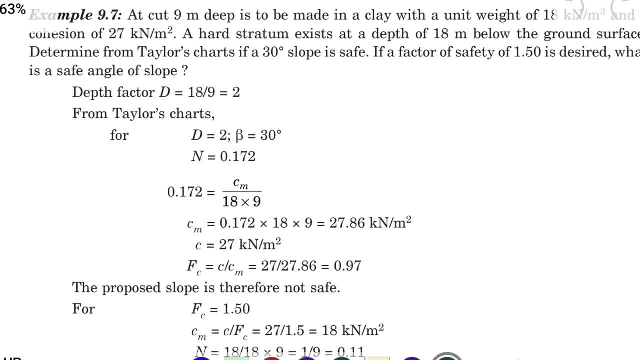 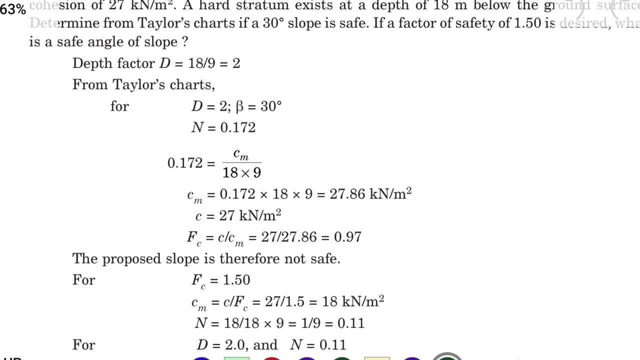 18. that is also given 18 kilo Newton per meter cube and h values 9, so the 9 meter deep, so we can substitute all the values, so cm equal to 0.172 into 18, into 9 equal to 27 point.